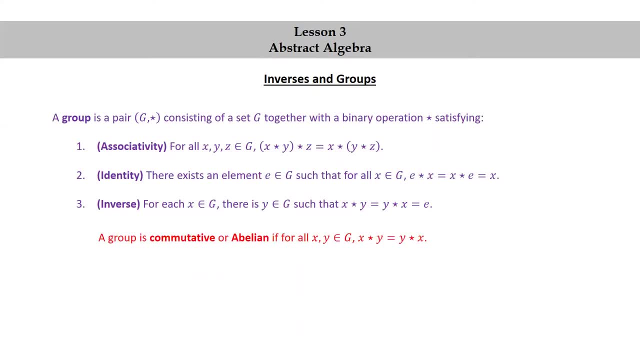 a group is commutative or abelian if for all x y and g x star y is equal to y star x let's look at an example is the commutative monoid z plus a group 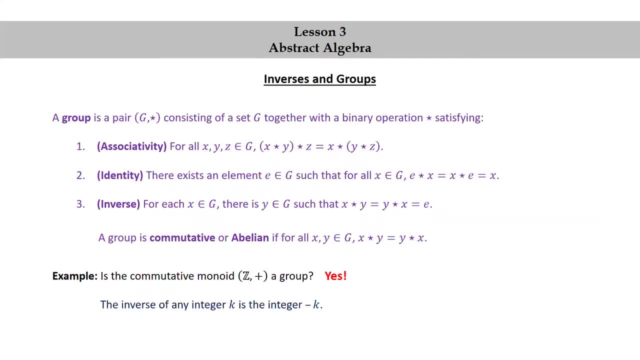 yes the inverse of any integer k is the inverse of any integer z plus a group then how is a group commutative or abelian if the commencement norm exposes itself to a n-tree transform is n-tree transform 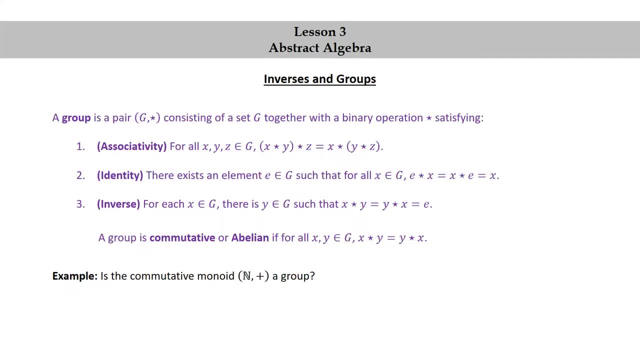 putting the strat千 or beinginary 수가 minus one by one zero point numbers then the null cube x and against zero point three comes the n-tree transformation over the in the set of natural numbers. 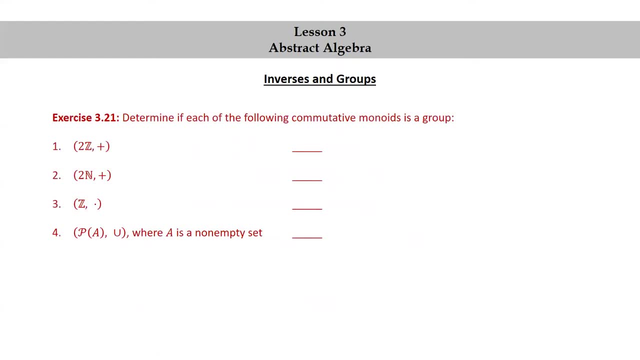 Let's try an exercise. Determine if each of the following commutative monoids is a group. Now's a good time to pause the video, try this exercise yourself, and then resume the video to check your answers against mine. Okay, 2z plus. Yes. The identity is zero and the inverse of 2k is negative 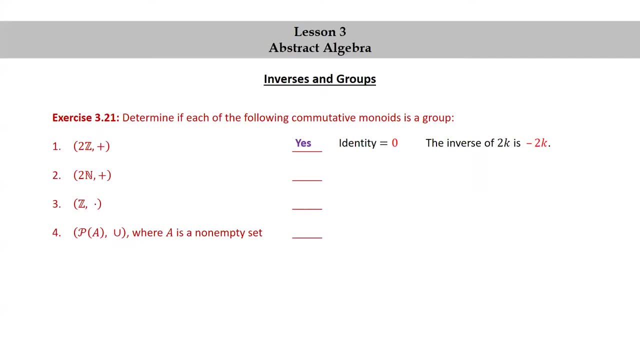 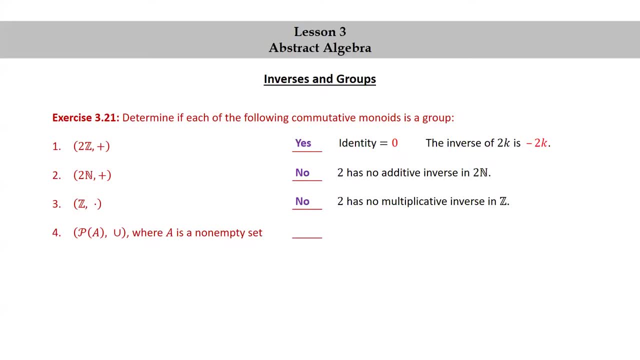 Power set of a together with union where a is a non-empty set. No. a has no inverse in the power set of a, for example. If b is in the power set of a, then since b is a subset of a, a union b is equal to a, which is not the empty set. Remember that the empty set is the identity of this commutative monoid. 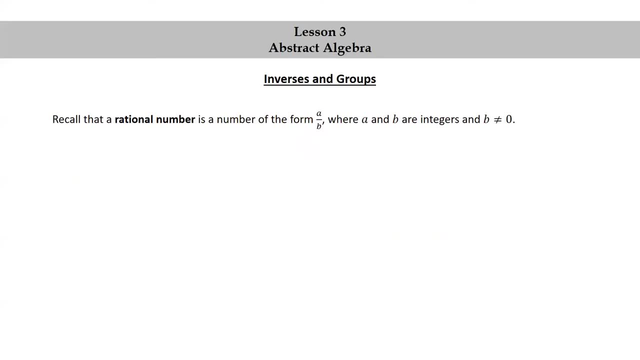 Recall that a rational number is a number of the form a over b, where a and b are integers and b is non-zero. We identify rational numbers a over b and c over d whenever ad is equal to bc. For example, 1 half and 3 sixths represent the same rational number because 1 times 6 is equal to 6 and 2 times 3 is equal to 6. We denote the set of rational numbers by double struck q. So we have q equal to the set of quotients a over b such that a and b are integers and b is not zero. We identify the rational number a over 1 with the integer a. 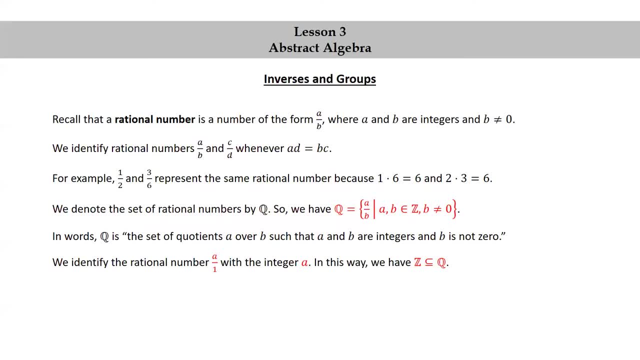 In this way, we have that the set of integers is a subset of the set of rational numbers. We add two rational numbers using the rule a over b plus c over d is equal to a times d plus b times c over b times d. Note that zero equals zero over one is an identity for the set of rational numbers together with addition. 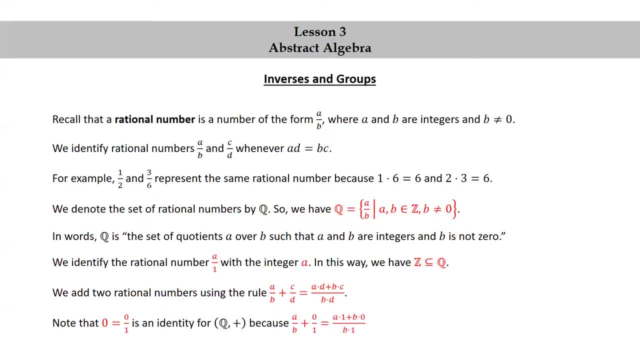 Because a over b is a set of integers and b is a subset of the set of rational numbers. a over b plus zero over one is equal to a times one plus b times zero over b times one which is a over b and zero over one plus a over b is equal to zero times b plus one times a over one times b which is also a over b. 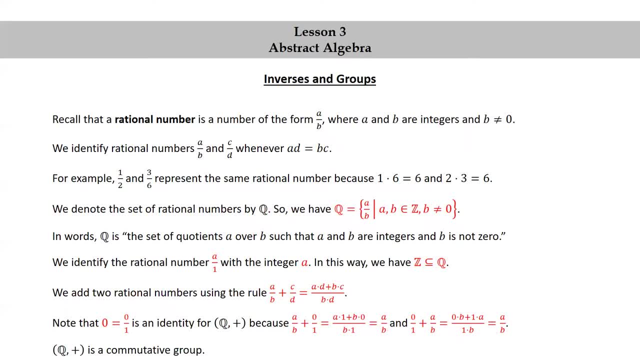 The set of rational numbers together with addition is a commutative group. 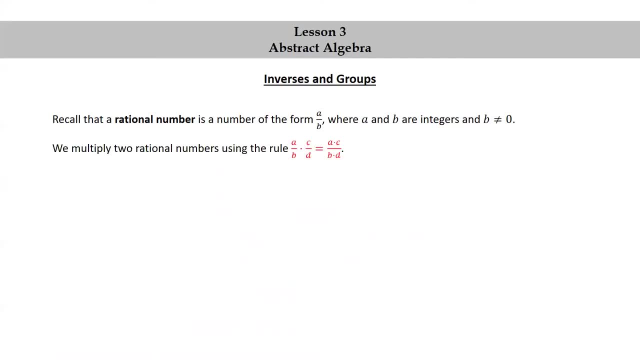 We multiply two rational numbers using the rule. a over b times c over d equals a times c over b times d. Note that 1 equals 1 over one is an identity for the set of rational numbers together with multiplication. Because a over b times one over 1 is a times 1 over b times 1 which is a over b. And one over one times a over b is one times a over one times b. times b which is also a over b. Now 0 times a over b is equal to 0 over 1 times a over b which is 0 times a over 1 times b which is 0 over b which is 0. In particular when we multiply 0 by any rational number we can never get 1. So 0 is a rational number with no multiplicative inverse. It follows that the set of rationals together with multiplication is not a group. However 0 is the only rational number without a multiplicative inverse. 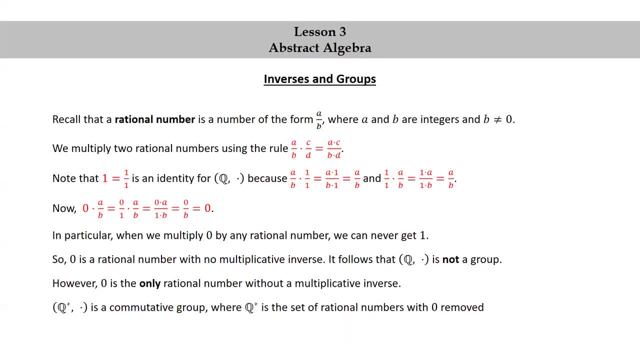 Q star together with multiplication is a commutative group where Q star is the set of rational numbers with 0 removed. 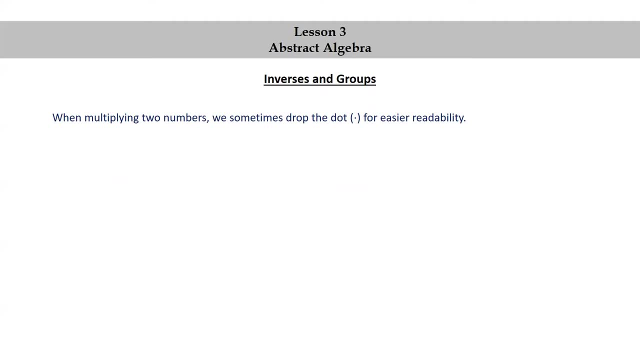 When multiplying two numbers we see that the set of rational numbers with 0 is 0. The otherok angle is a constant of q lines. 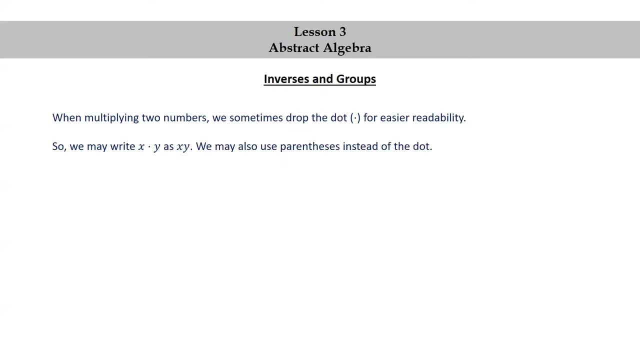 Can we simplify this into a theoretical hypothesis? 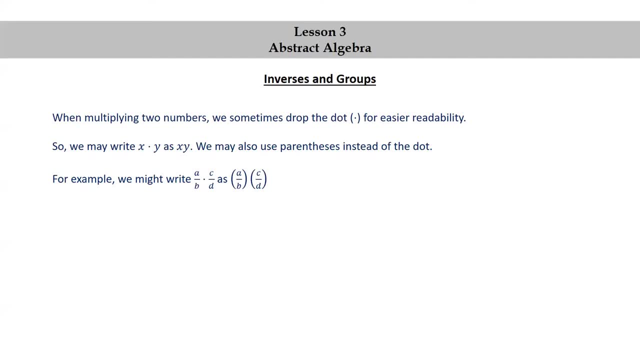 A plot of siamofrequencies means that the kill numbers are not slog on the plot line. 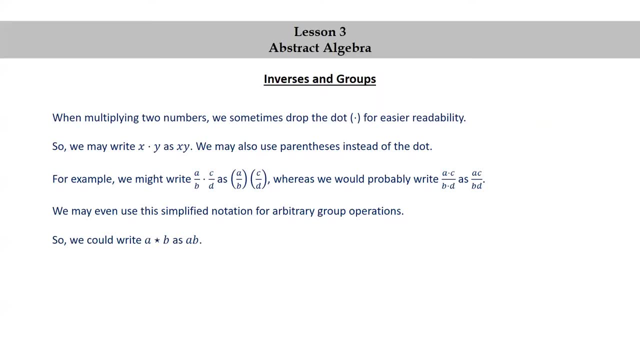 for arbitrary group operations. So we could write A star B as AB. However, we will avoid doing this if it would lead to confusion. For example, we will not write A plus B as AB. That would just be confusing. Let's try another exercise. Let 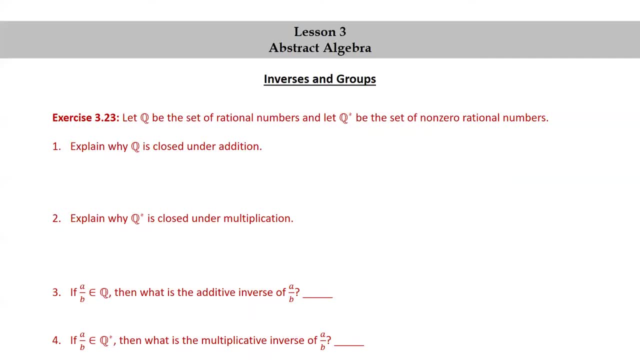 Q be the set of rational numbers and let Q star be the set of non-zero rational numbers. Go ahead and pause this video. Try this exercise yourself and then resume the video to check your answers against mine. 1. Explain why Q is closed under addition. Let A over B and C over D be in Q. Then that means that A B 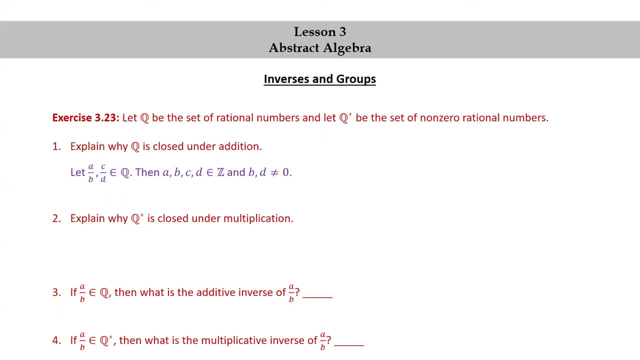 C and D are in Z set of integers and B and D are nonzero. Since the подход set of bound them against a Level Q family, let's do the following block. Since the subject set explicitly states B as an alternative and theTR set as an acabou viola de original numuma, Хотя a break in Cy overview- winning okay but talking about who is dispos h お rappersiți? Dever입니다. Leperaanți. The final question is, how does the of integers is closed under multiplication, ad, bc, and bd are all integers. Since the set of integers is closed under addition, ad plus bc is an integer. Since b and d are non-zero, 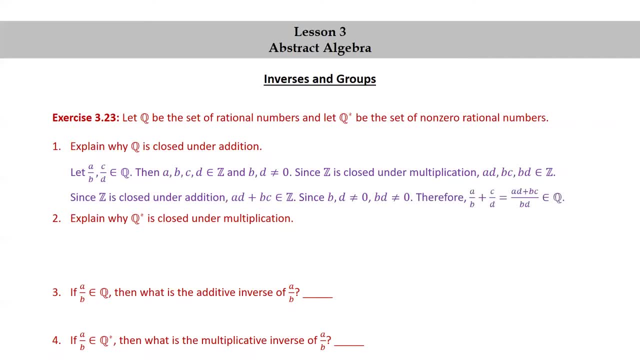 b times d is non-zero. Therefore a over b plus c over d is equal to ad plus bc over bd is a rational number. Okay now number two. Let's explain why q star is closed under multiplication. 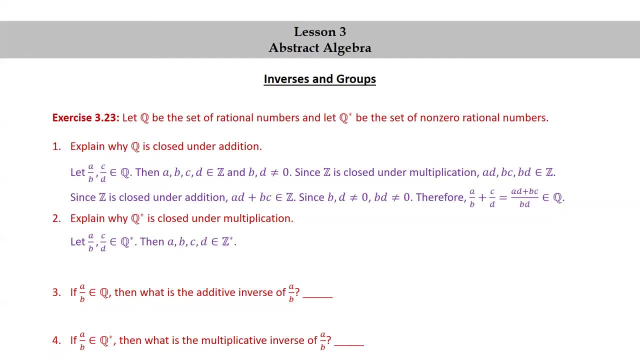 Let a over b c over d be in q star then a b c and d are in z star, they're all non-zero integers. Since z star is closed under multiplication ac and bd are both in z star, therefore a over b times c over d is equal to a. d is equal to ac over bd is in q star. 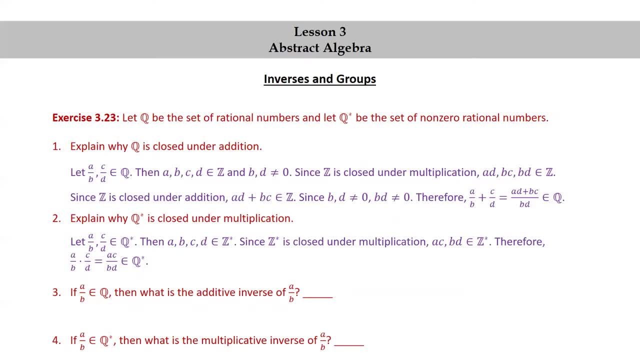 Okay third one, if a over b is in q then what is the additive inverse of a over b? It's negative a over b. And for number four, if a over b is in q star what is the multiplicative inverse of a over b? That's b over a. 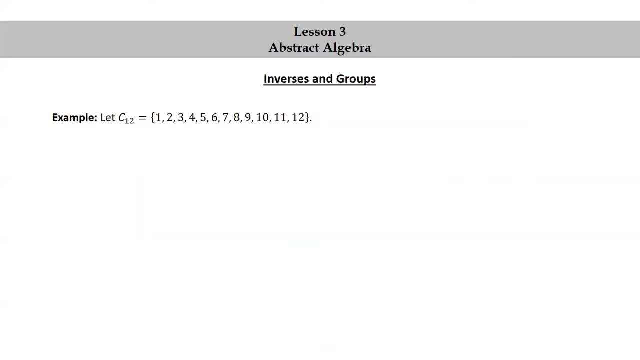 It's time for another example. Let c12 be the set consisting of the numbers from 1 through 12. 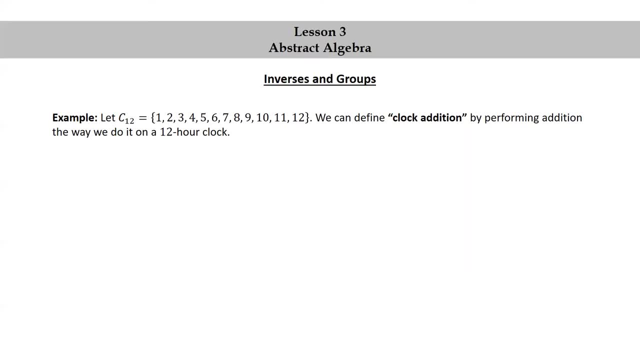 We can define clock addition by performing addition the way we do it on a 12-hour clock. Here's a picture of a 12-hour clock. Let's do a couple of computations. 3 plus 5 is equal to 8, right? Because if it's 3 o'clock now then 5 hours later it will be 8 o'clock. 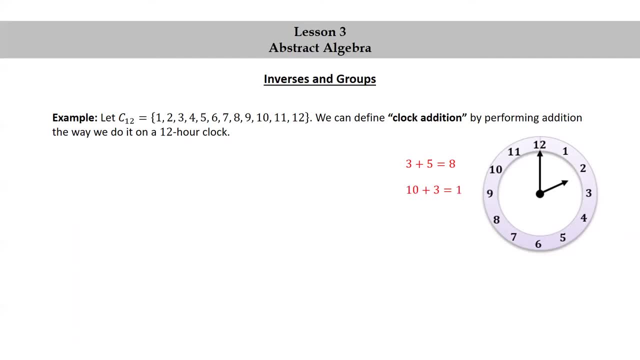 And 10 plus 3 is equal to 1 because if it's 10 o'clock now then in 3 hours it'll be 1 o'clock, right? 10, 11, 12, 1. 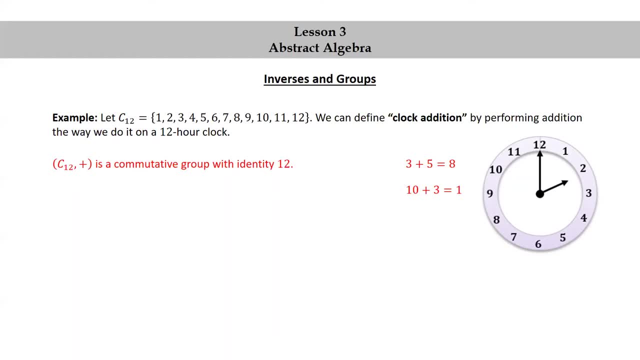 c12 together with clock addition is a commutative group with identity 12. 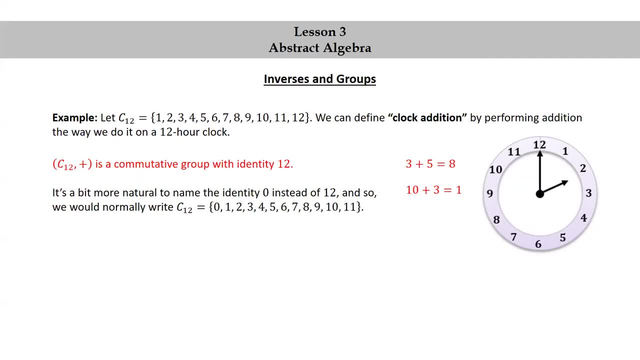 It's a bit more natural to name the identity 0 instead of 12 and so we would normally write c12 as the set of, numbers from 0 through 11. So I'll just replace that 12 by a 0 on the clock. 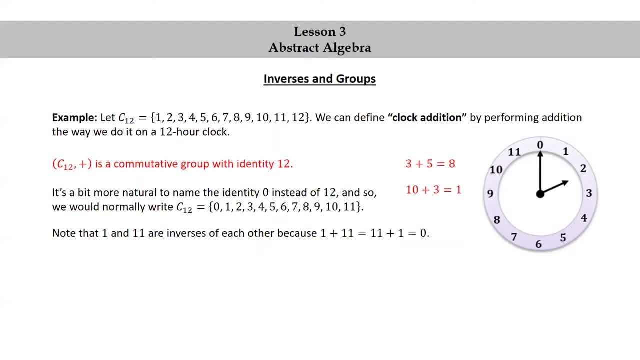 Note that 1 and 11 are inverses of each other because 1 plus 11 and 11 plus 1 are both equal to 0. Similarly we have the following pairs of inverses 2 and 10, 3 and 9, 4 and 8 and 5 and 7. 5 and 7. 5 and 7. 6 and 7. 5 and 7. Also 0 and 6 are inverses. 6 and 6 are inverses. 6 and 6 are inverses. 4 and 4 are inverses. 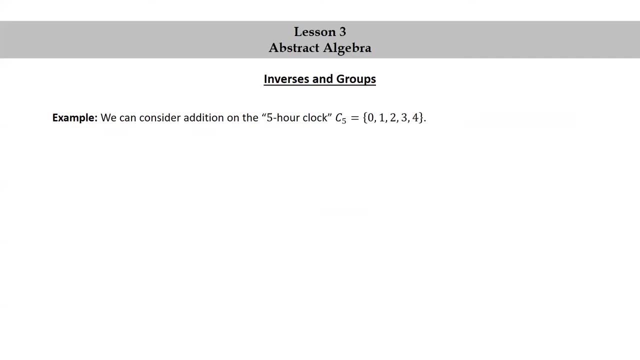 We can consider addition on the 5-hour clock, c5 equals the set consisting of 0, 1, 2, 3, and 4. 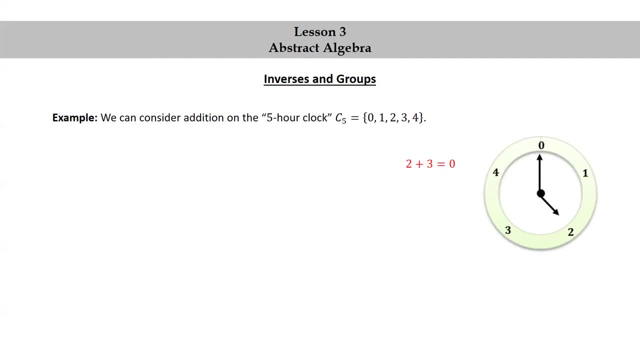 Here's a picture of a 5-hour clock. For example, 2 plus 3 is 0, and 3 plus 4 is 2. 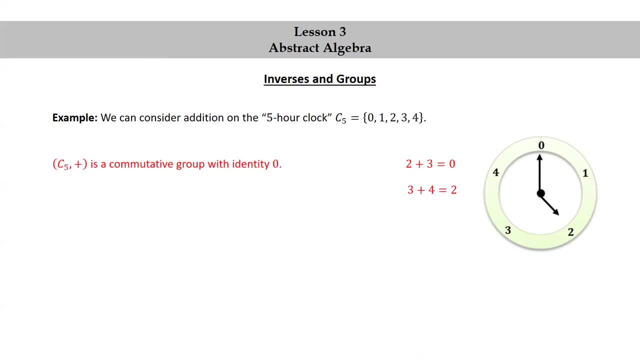 c5 together with addition is a commutative group with identity 0. We have the following inverse pairs, 1 and 4, and 2 and 3. 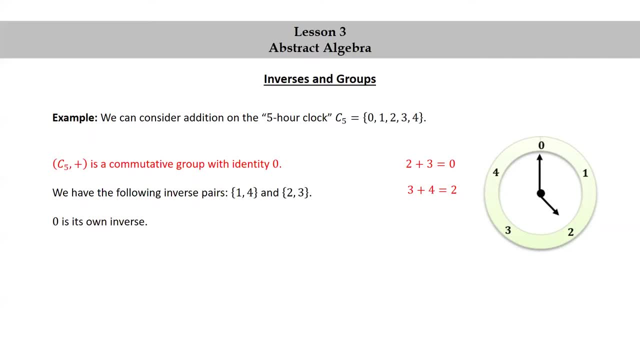 Also 0 is its own inverse. 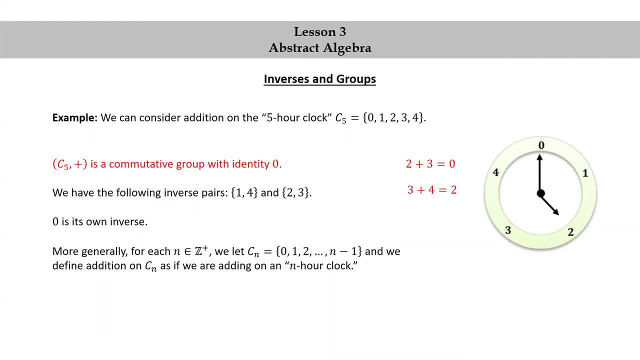 More generally, for each positive integer n, we can let c sub n be the set of 0 through n minus 1, and we define 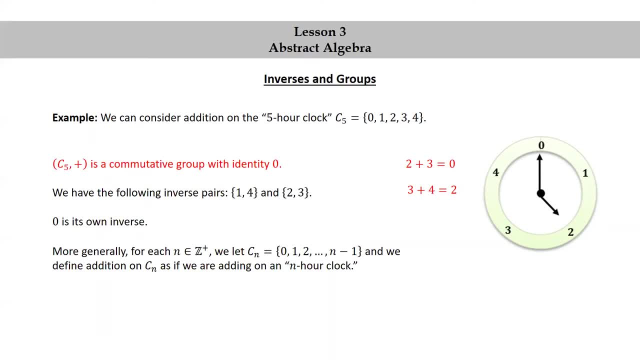 addition on c sub n as if we were adding on an n-hour clock. c sub n together with addition is always a commutative group with identity 0. 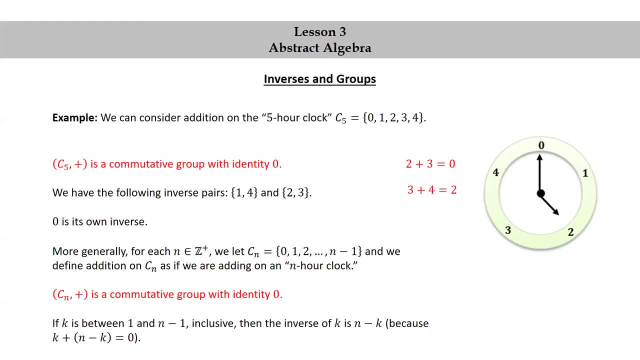 If k is between 1 and n minus 1 inclusive, then the inverse of k is n minus k. 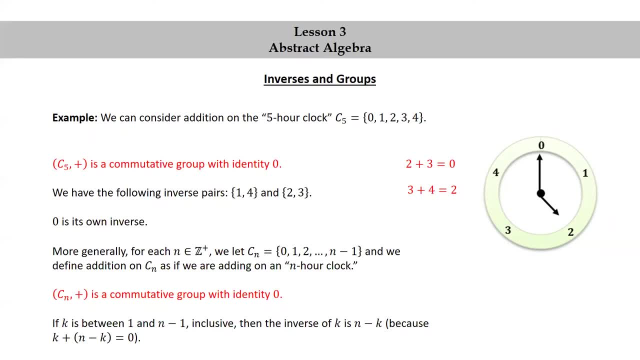 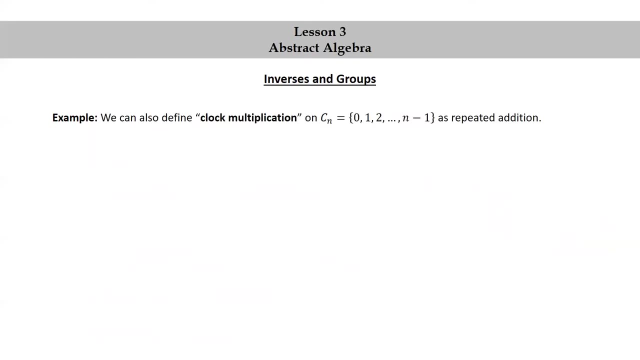 So when we add k plus n minus k, we get n, which is the same thing as 0 on the clock. The inverse of 0 is 0. We can also define clock multiplication on cn as repeated addition. For example, on c12 we have 2 times 5 is equal to 5 plus 5 is 0. Right? So, when we add k plus n minus k, we get n, which is the same thing as 0 on the clock. Inperseptitive this set of 0 through n minus 1 for lucky boxes. Now let's look at it in theses stuffed numbers. 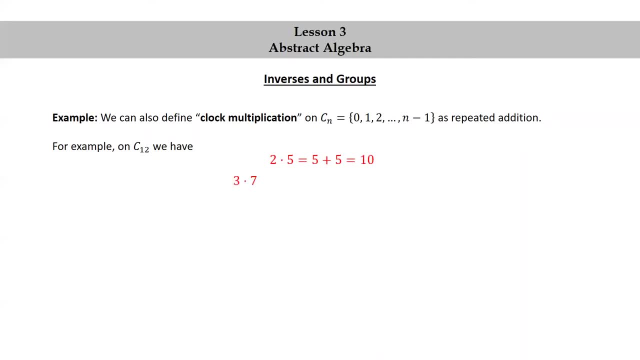 o and o. podemdoem Bohemen is equal to 0 for different sum numbers and the exact number number for any number. 5 which is 10. As another example 3 times 7 is equal to 7 plus 7 plus 7 which is 2 plus 7 right because 7 plus 7 is 2 on a 12 hour clock and 2 plus 7 is 9. We can also perform this last computation by multiplying 3 and 7 as we would normally to get 3 times 7 equals 21 and then subtracting 12 because we're on a 12 hour clock to get 21 minus 12 equal to 9. Notice we get the same answer. 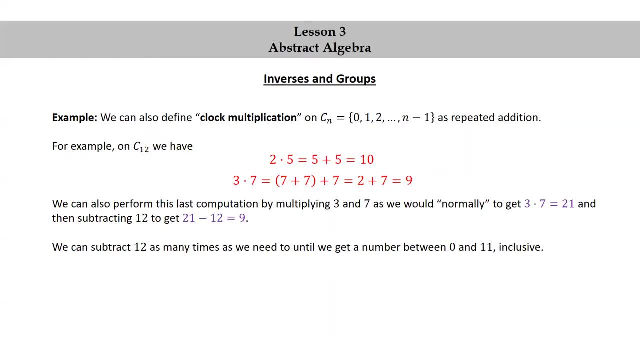 We can subtract 12 as many times as we need to until we get a number between 0 and 11 inclusive. For example 5 times 8 is equal to 40 and subtracting 12 three times from 40 gives us a result of 40 minus 36 right the 36 is because 12 times 3 is 36 and we get 4. So 5 times 8 is equal to 4 on a 12 hour clock. We can also perform this computation more quickly by taking the remainder upon dividing 40 by 12. Indeed 12 goes into 40 three times with a remainder of 4. 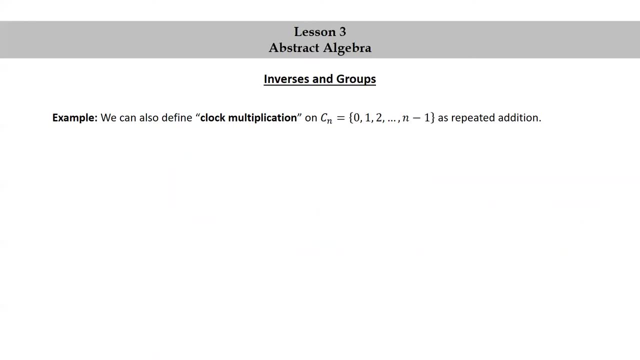 cn together with multiplication where cn as usual is the set of 0 through n minus 1 and we define clock multiplication as repeated addition. This gives us a commutative monoid with identity 1. However for each n in z plus 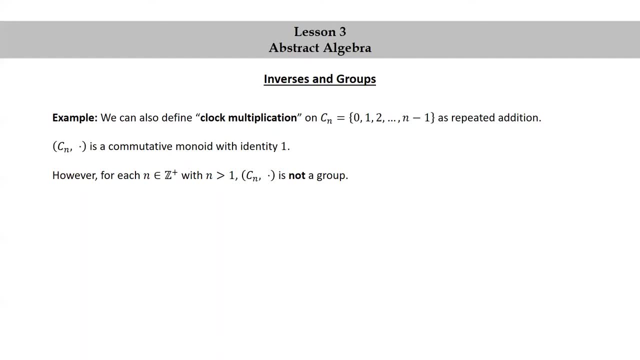 with n greater than 1 cn together with multiplication is not a group. 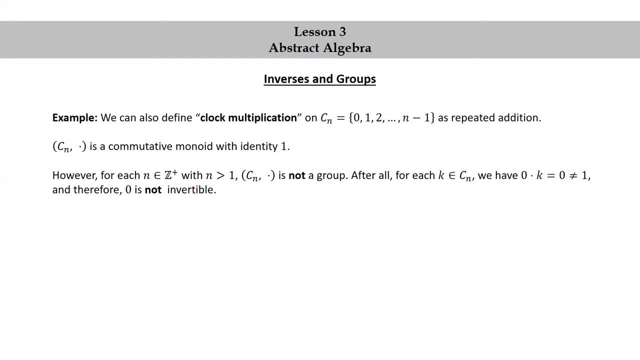 After all for each k in cn we have 0 times k is equal to 0 which is not equal to 1 and therefore 0 is not invertible. For some values of n if we remove 0 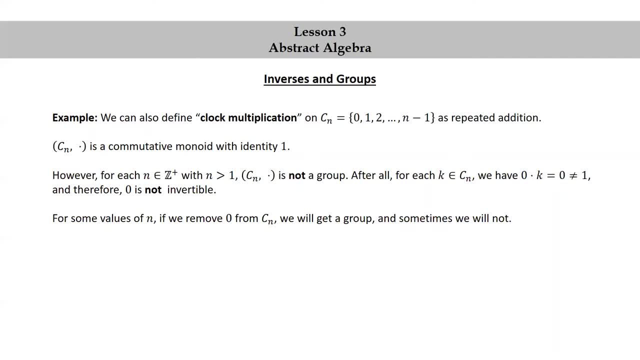 from cn we will get a group and sometimes we will not. For example c3 minus 0 together with clock multiplication or the set consisting of 1 and 2 together with clock multiplication is a group. Where the operation is 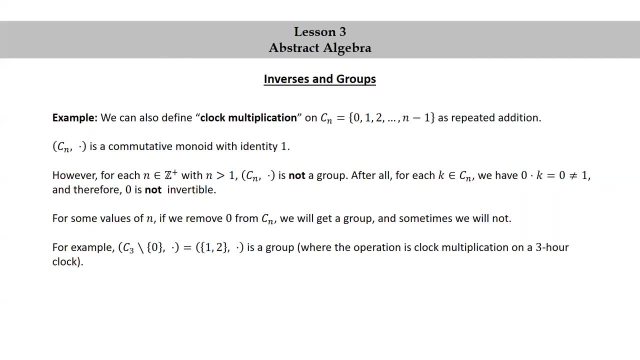 clock multiplication on a 3 hour clock. 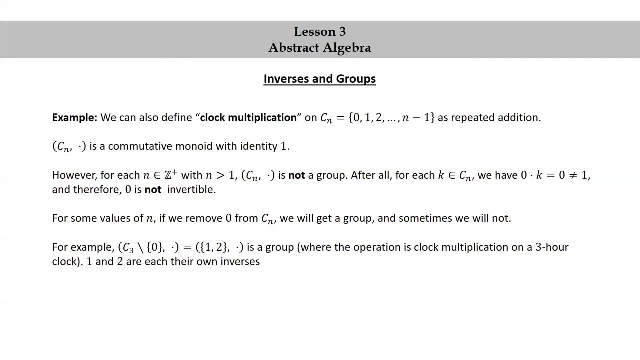 1 and 2 are each their own inverses right. 1 times 1 is 1 and 2 is 2 plus 2 which is 4 but on a 3 hour clock that's equal to 1. 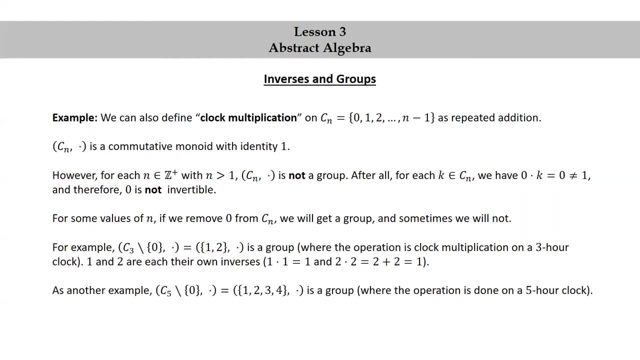 As another example c5 was 0 removed together with clock multiplication the setpot used is 10 times recognize 0 is 420 is 2. 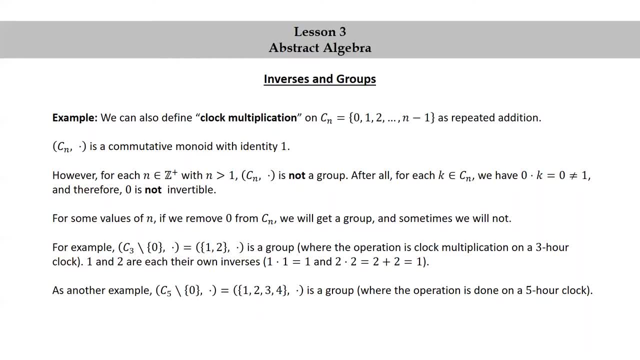 with clock multiplication is uh well that's the set consisting of one two three and four together with clock multiplication is a group where we're doing this on a five hour clock 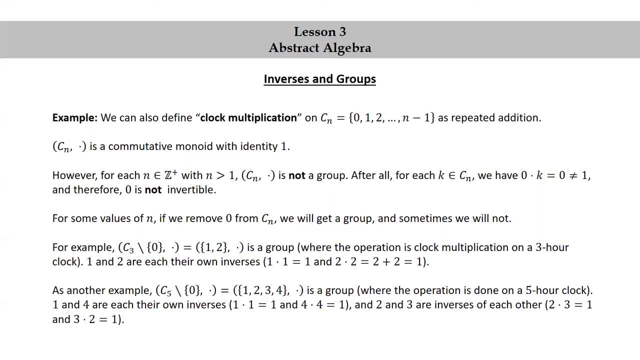 one and four each their own inverses one times one is one and four times four is 16 which is the same as one on a five hour clock and two and three are inverses of each other because two times 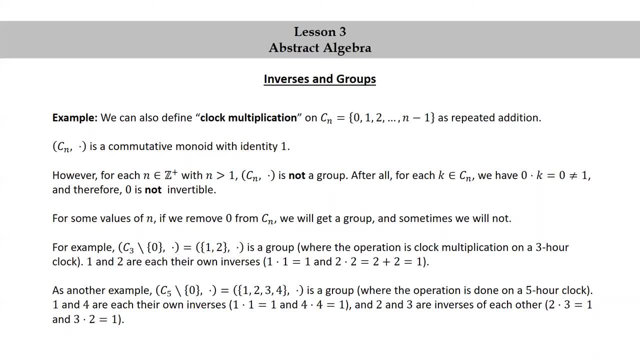 three and three times two are both six which is the same as one on a five hour clock 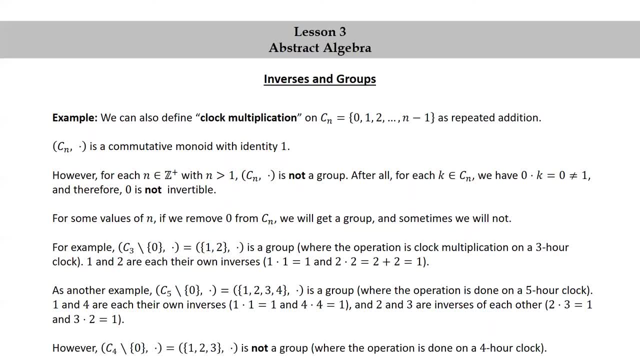 however c4 with zero removed together with clock multiplication the set of one two three together with clock multiplication is not a group here the operation is being done on a four hour 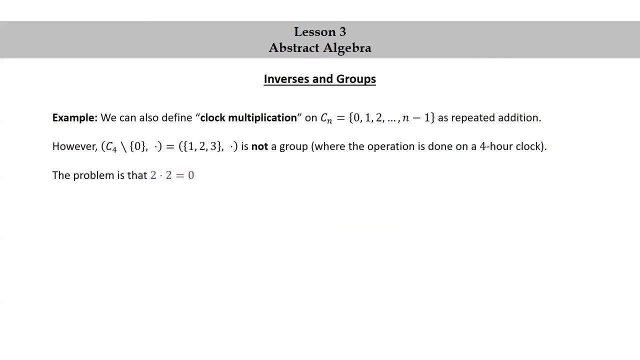 clock the problem is that two times two is equal to zero and so the partial binary operation of 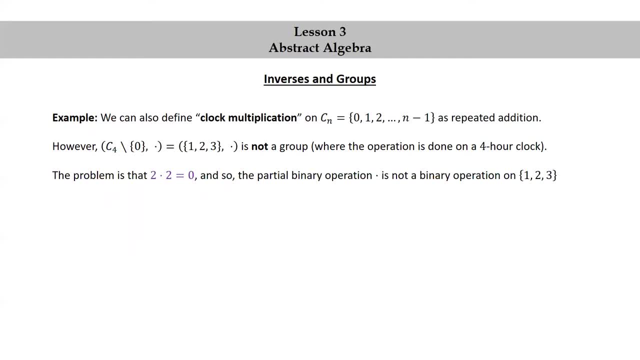 clock multiplication is not a binary operation on the set consisting of 1, 2, and 3. 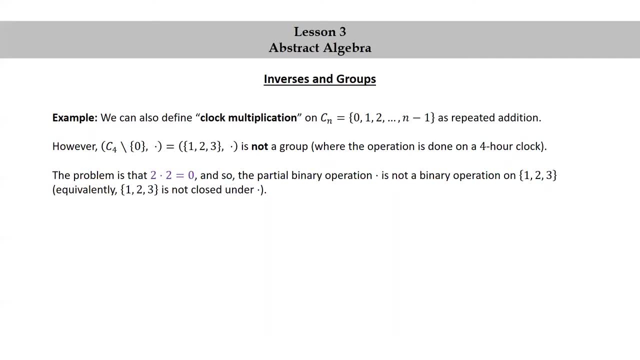 Equivalently, the set consisting of 1, 2, and 3 is not closed under clock multiplication on a 4-hour clock. If we delete the offending element 2 from this set, we see that the set consisting of 1 and 3, together with clock multiplication on a 4-hour clock, is a group. 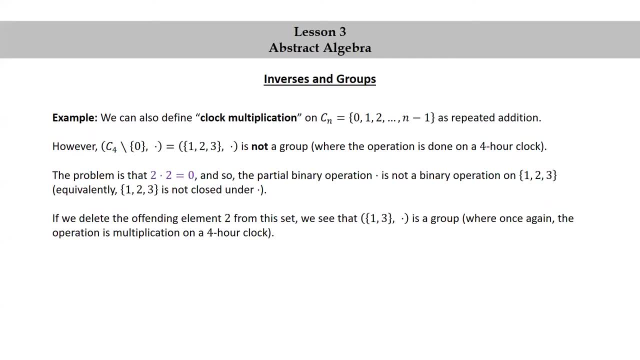 Okay, once again, the operation is multiplication on a 4-hour clock. 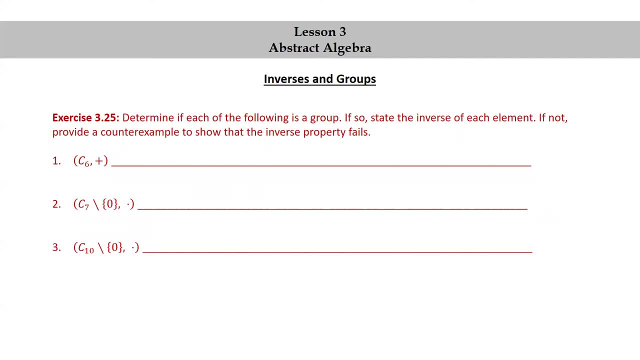 Let's try another exercise. Determine if each of the following is a group. If so, state the inverse of each element. If not, provide a counterexample to show that the inverse property fails. Okay, now's a good time to pause the video, try these problems yourself, and then resume the video to check your answers against mine. 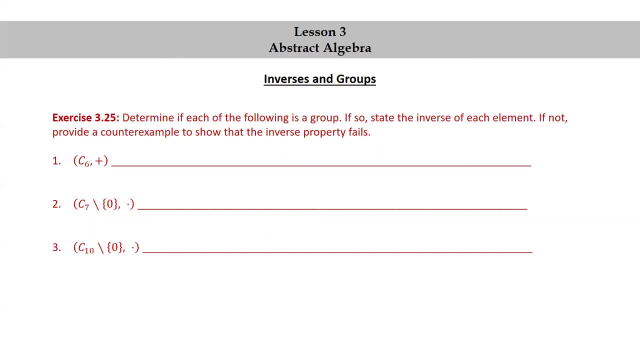 Okay, the first one, C6, together with clock addition, yes, this is a group. The inverse pairs are 0 is paired with itself, 1 and 5, 2 and 4, and 3 is paired with itself. 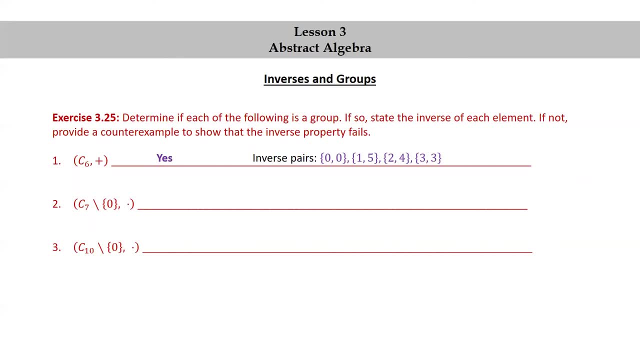 C7 with 0 removed under clock multiplication, yes, the inverse pairs are 1 is paired with itself, 2 and 4, 3 is paired with 5, and 6 is paired with itself. In this case, the inverse pairs are 0 is paired with itself. 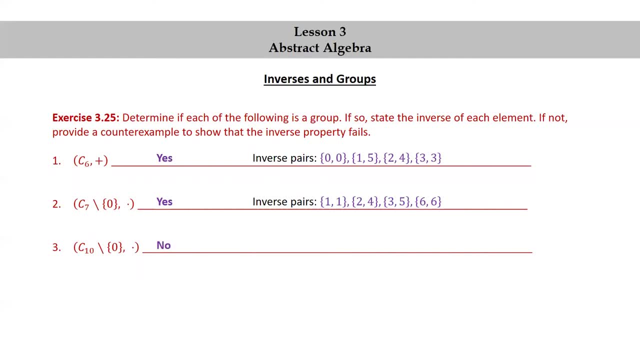 C10 with 0 removed under clock multiplication, for this one, the answer is no. 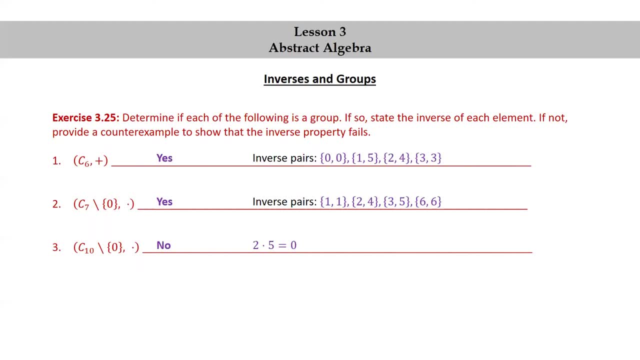 The problem is that 2 x 5 is equal to 0 on a 10-hour clock. So if 2-inverse were to exist, then 5 could be written as 1 x 5, and then 1 would be able to be written as 2 inverse times 2 by the inverse property. 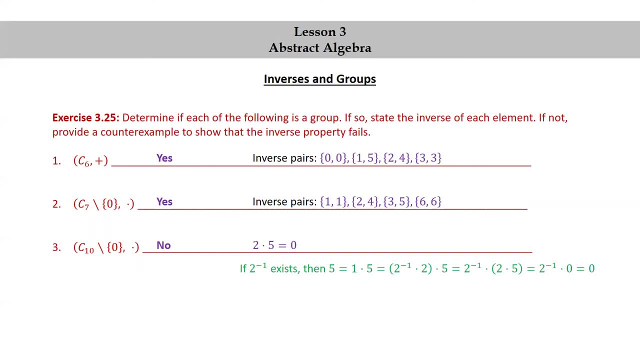 Then we could use associativity. to write 2 inverse times 2 times 5 as 2 inverse times 2 times 5, but 2 times 5 is 0, so we get 2 inverse times 0, which is 0. 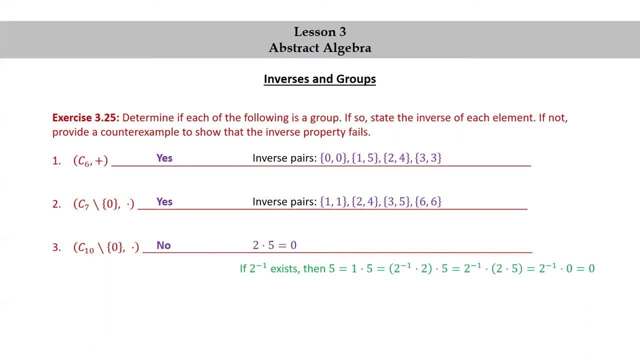 This would show that 5 would be equal to 0, which is not true. Let's look at another example. 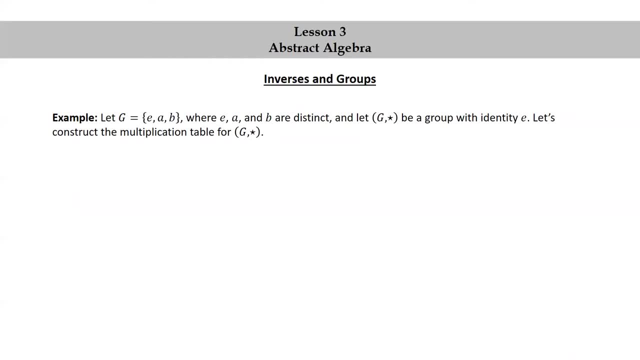 Let G be the set consisting of E, A, and B, where E, A, and B are distinct, and let G star be a group with identity E. For E, let's construct the multiplication table for G star. 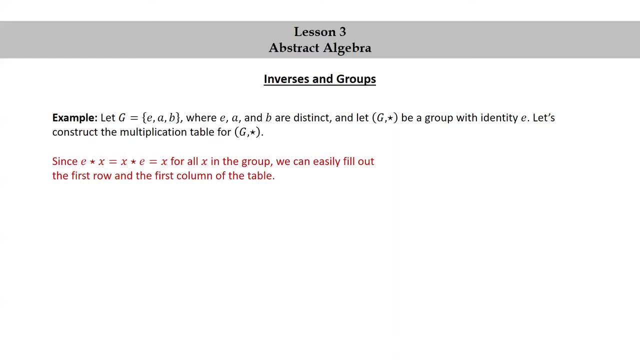 Since E star X is equal to X star E is equal to X for all X in the group, because E is an identity, 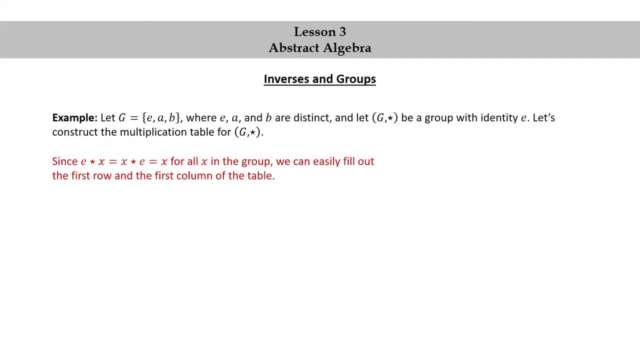 we can easily fill out the first row and the first column of the table. In other words, we can just copy the input row to the row corresponding to E, and we could copy the input column to the column corresponding to E to already get 5 of the elements. 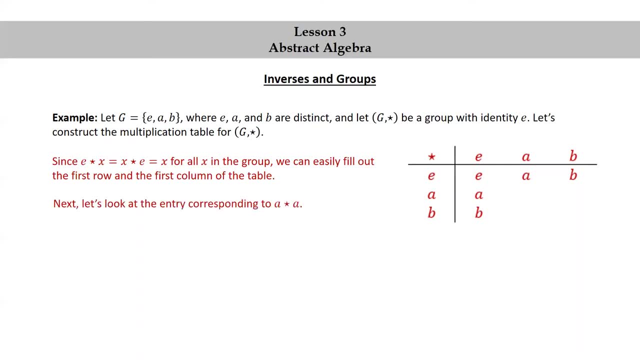 Next, let's look at the entry corresponding to A star A. I'll denote that with a box with a dot in it, a dotted box. Note that the same element cannot appear twice in any row. 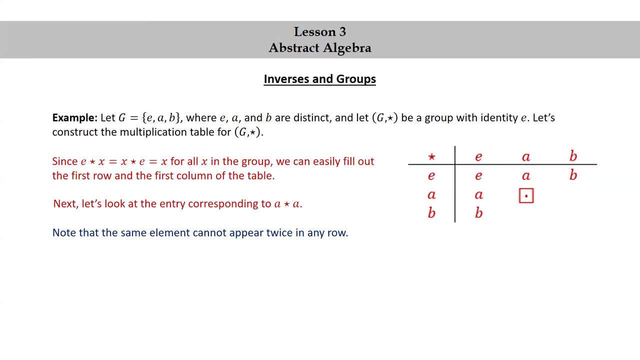 Let me give a brief explanation as to why that's true. However, this may be a little confusing, so if you don't understand it or you have a little trouble with it and need some time to work it out, for now you could just accept the fact that the same element cannot appear twice in any row. 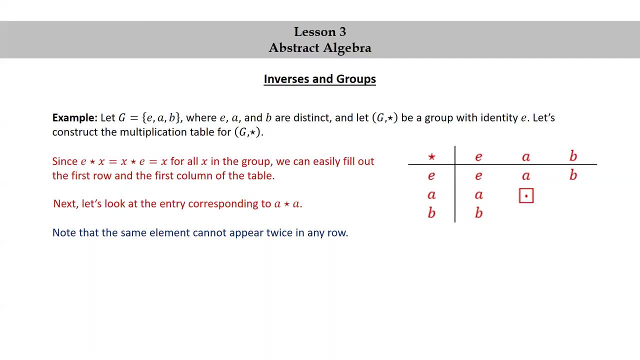 You don't have to sit and struggle with this explanation if you don't want to, but I'm going to provide it for completeness. 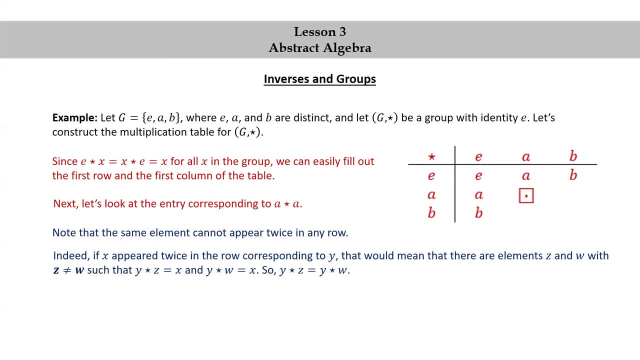 So indeed, if X appeared twice in the row corresponding to Y, that would mean that there are elements Z and W with Z not equal to W, such that X star Z is equal to X and Y star W is equal to X. 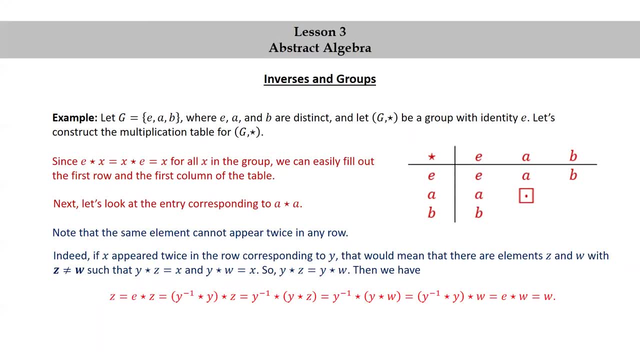 So Y star Z is equal to Y star W. Then we have Z could be written as E star Z, which could be written as Y inverse star Y star Z. We could then use associativity to write that as Y inverse star Y star Z. We could replace the Y star Z with Y star W to get Y inverse star Y star W. Using associativity, we get Y inverse star Y star W, which is E star W using the inverse property, and that's equal to W. So we have that Z is equal to W here, which, you know, they're supposed to be the same. 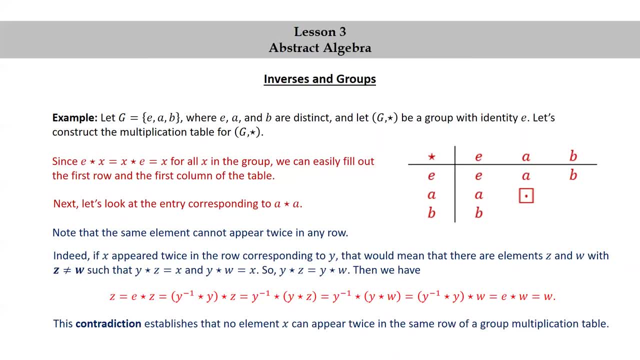 They're supposed to be distinct. This contradiction establishes that no element X can appear twice in the same row of a group multiplication table. 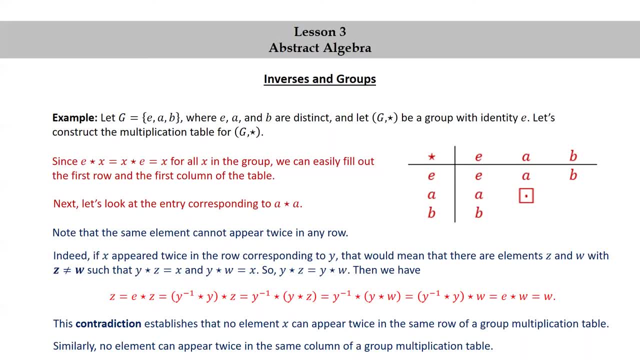 Similarly, no element can appear twice in the same column of a group multiplication table. 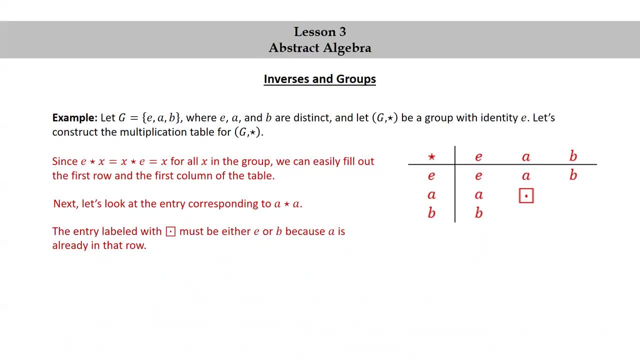 The entry labeled with the dotted box must be either E or B because A is already in that row. If it were E, then the final entry in the row would be a B, giving two Bs in the last column. 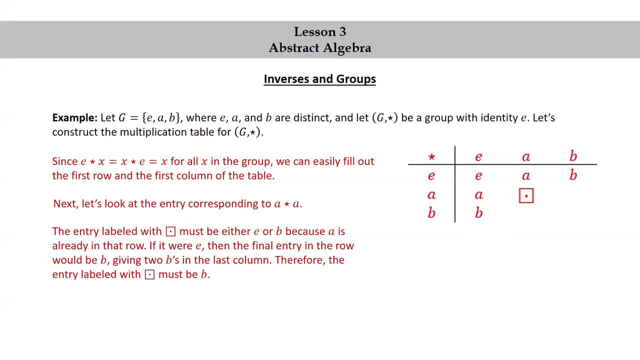 That's a problem. Therefore, the entry labeled with the dotted box must be B. 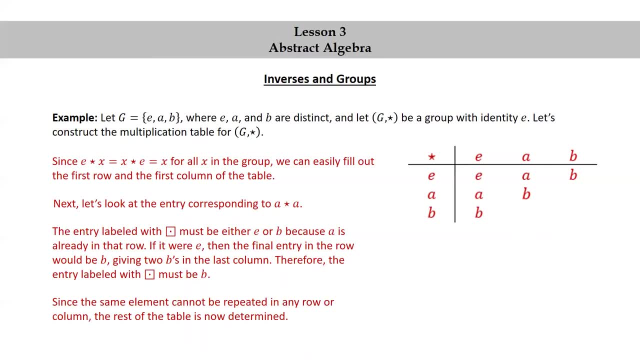 Since the same element cannot be repeated in any row or column, the rest of the table is now determined. In the second row, we have an A and B, so that must be followed by an E. In the second column, we have AB, so that must be followed by E. And then we could use either the third row or the third column to see we have BE followed by A. 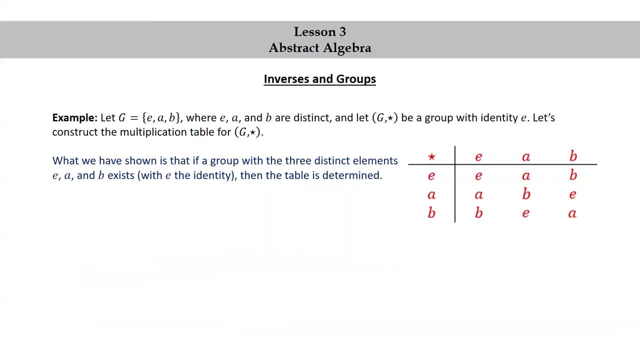 What we have shown is that if a group with the three distinct elements E, A, and B exists with E, B identity, then the table is determined. 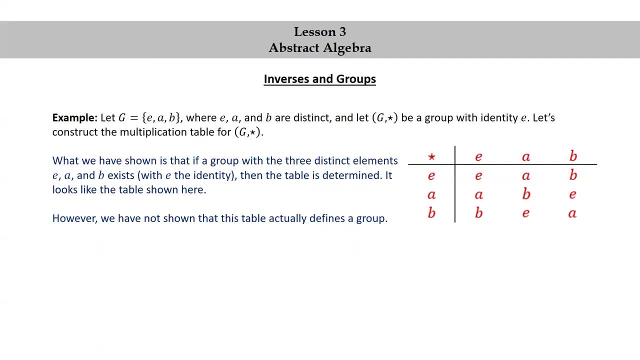 It looks like the table shown here. However, we have not shown that this table actually defines a group. 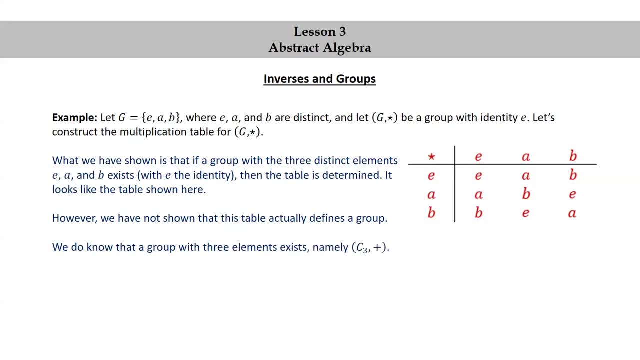 We do know that a group with three elements exists, namely C3, together with clock addition. If we replace E, A, and B with 0, 1, and 2 respectively, and the operation star with clock addition, we get the table for C3+. 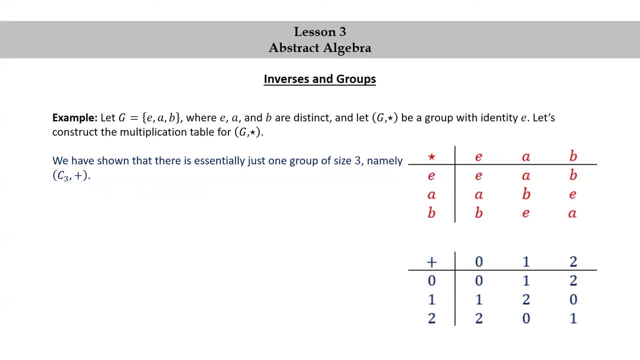 We have shown that there is essentially just one group of size 3, namely C3, together with clock addition. Any other group with three elements will look exactly like this one, except for possibly the names of the elements. 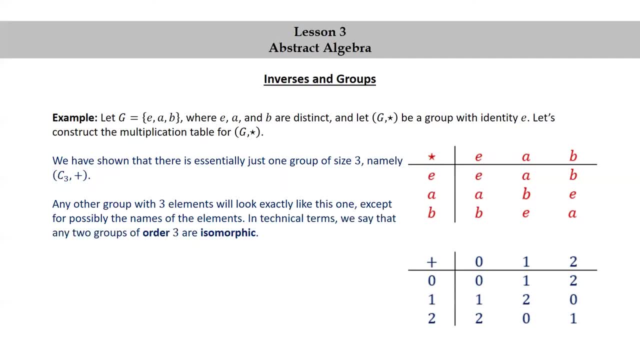 In technical terms, we say that any two groups of order 3 are isomorphic. The order of a group is just the number of elements in the group. 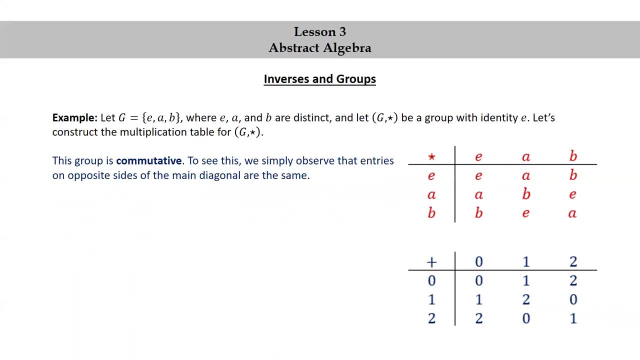 This group is commutative. To see this, we simply observe that entries on opposite sides of the main diagonal are the same. 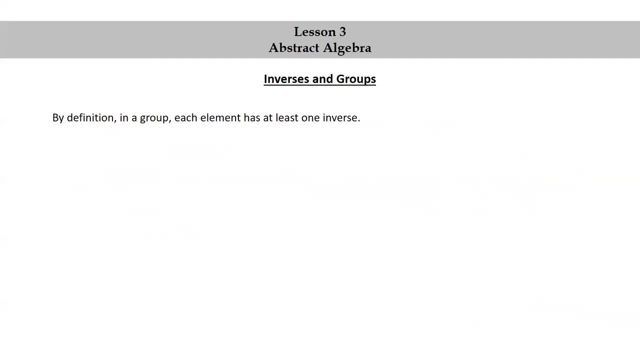 By definition, in a group, each element has at least one inverse. It is natural to ask if a given element in a group can have more than one inverse. As it turns out, this cannot happen. 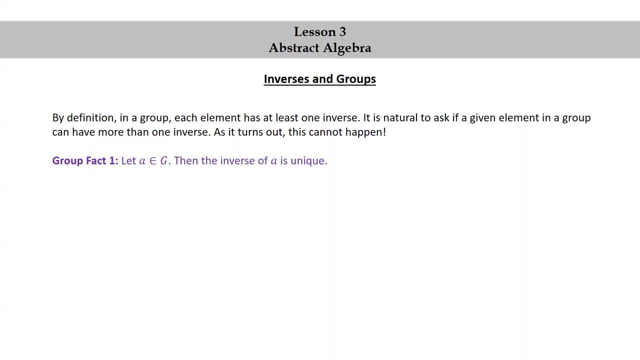 Group fact 1. Let A be in G, then the inverse of A is unique. Group fact 2. 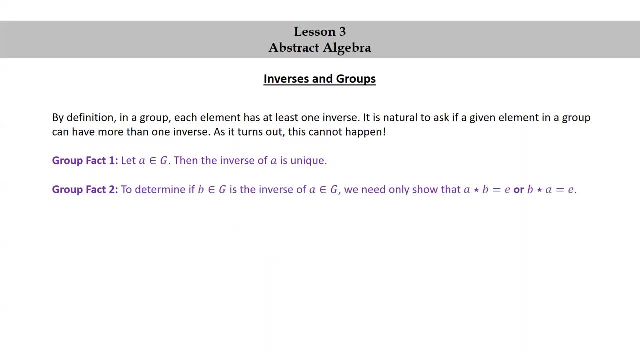 To determine if B in G is the inverse of A in G, we need only show that A star B equals E, or B star A equals E. 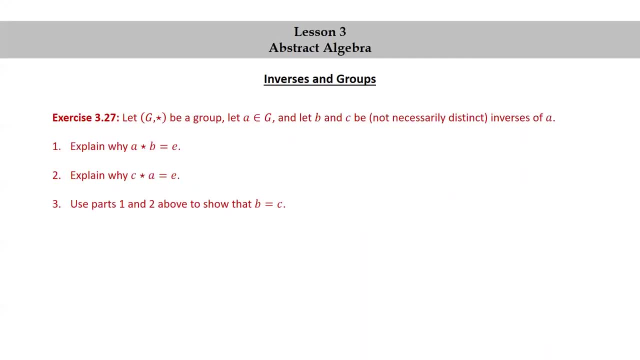 Let's finish one more exercise. Let G star be a group, let A be in G, and let B and C be not necessarily distinct inverses of A. Go ahead and pause the video, try this exercise, and then resume the video to check your answers against mine. 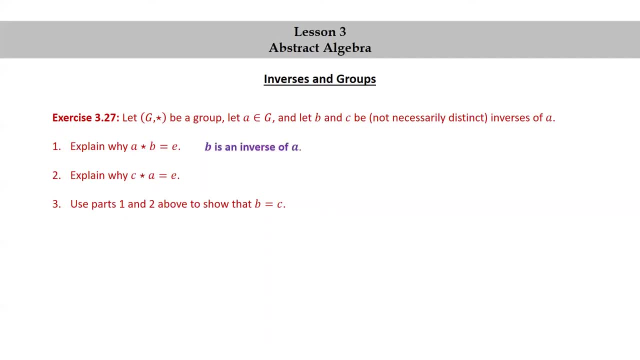 Explain why A star B is equal to E. This is because B is an inverse of A. 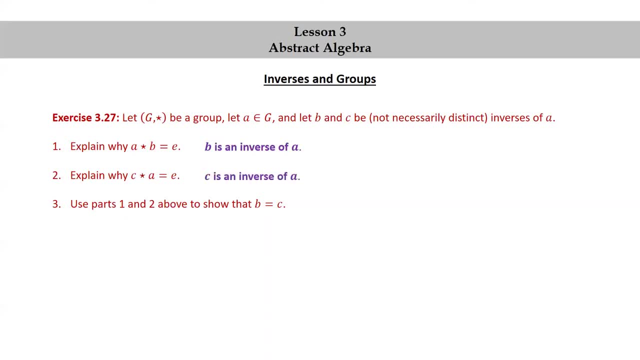 Explain why C star A is equal to E. This is because C is an inverse of A. 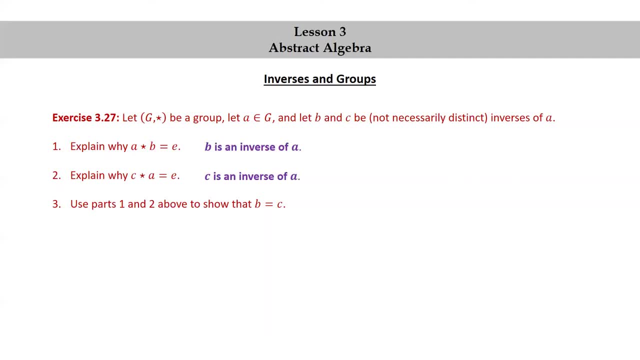 Use parts 1 and 2 above to show that B is equal to C. We have B equal to E star B using the identity property. And we could write E as C star A from 2. 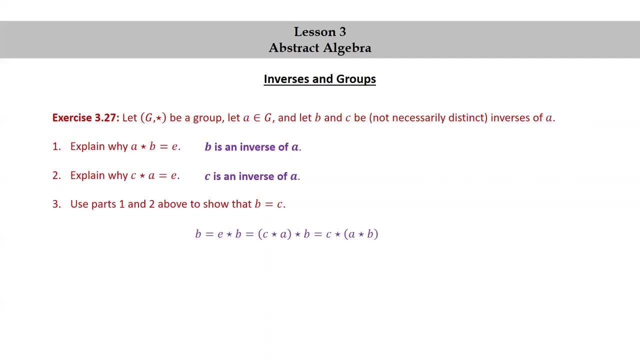 And then we could use associativity to write C star A star B as C star A star B. And then we could replace A star B with E from number 1 to get C star E. And C star E is just equal to C. So we see that we have shown that B is equal to C.